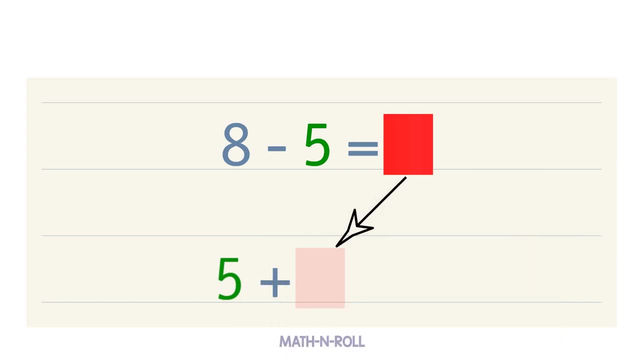 We had 8 minus 5 equals blank, and now we have 5 plus blank equals 8.. Let's use the model to solve the addition fact. We have 5 pieces. How many pieces do we add to make 8? 1,, 2,, 3.. We add 3 pieces to make 8.. We can use the addition fact to solve for the blank: 8 minus 5 equals blank. We can use the addition fact to solve for the blank: 8 minus 5 equals blank. We can use the addition fact to solve for the blank. 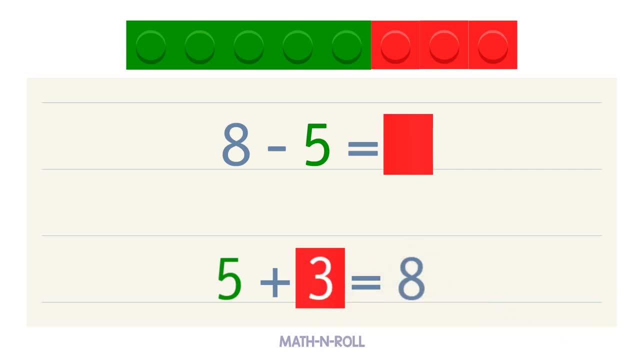 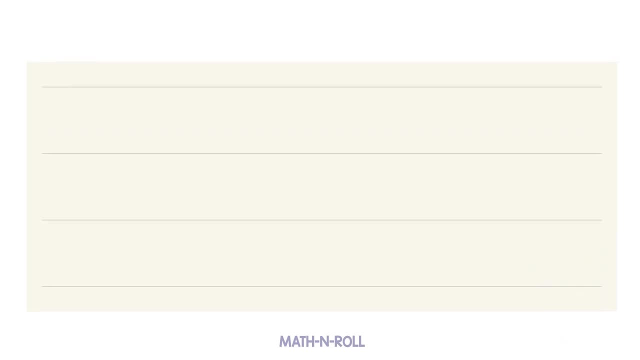 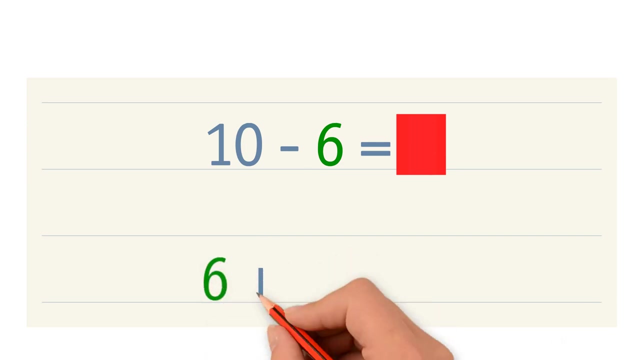 So 5 plus 3 equals 8.. 3 is our blank, So 8 minus 5 equals 3.. Let's do another example: 10 minus 6 equals blank. Let's write our related addition fact: 6 plus blank equals 10.. 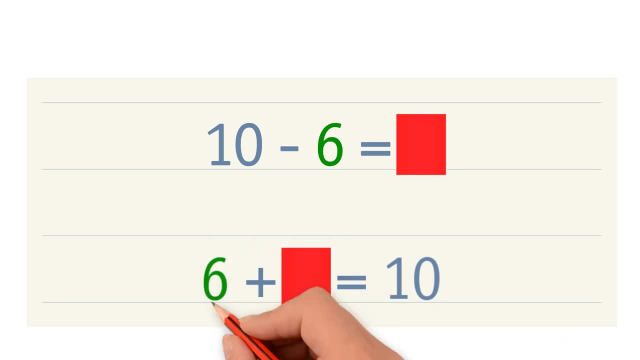 Use a multiple: 6 plus blank equals 10.. Let's use the model to solve the addition fact. We have 6 green pieces. How many more pieces do we need to make 10?? 1,, 2,, 3, 4.. We needed 4 more pieces to make 10.. So 6 plus 4 equals 10.. 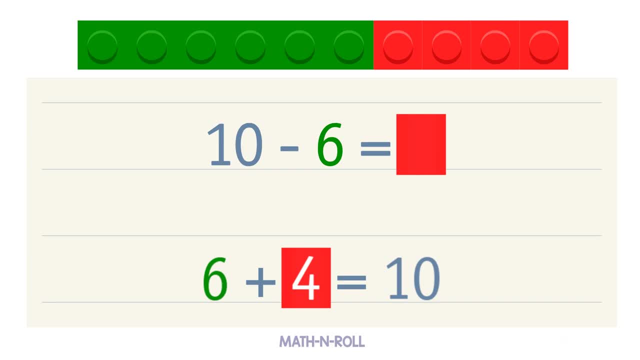 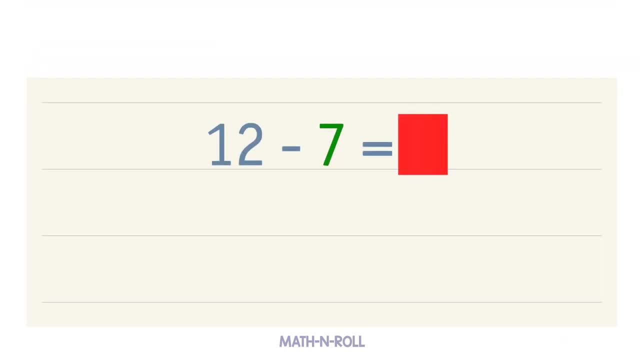 4 is our blank. So 10 minus 6 equals 4.. Let's do another one: 1. 12 minus 7 equals blank. Write the related addition fact: 7 plus blank equals 12.. Use the model to solve. We have 7 green circles. 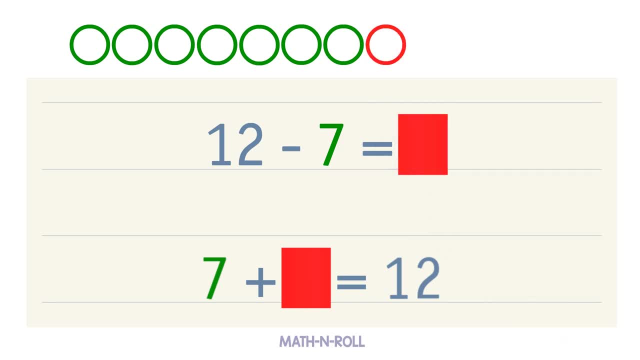 How many more circles do we need to make 12?? 1,, 2,, 3,, 4, 5.. We needed 5 more circles to make 12, so 7 plus 5 equals 12.. 5 is our blank, so 12 minus 7 equals 5..